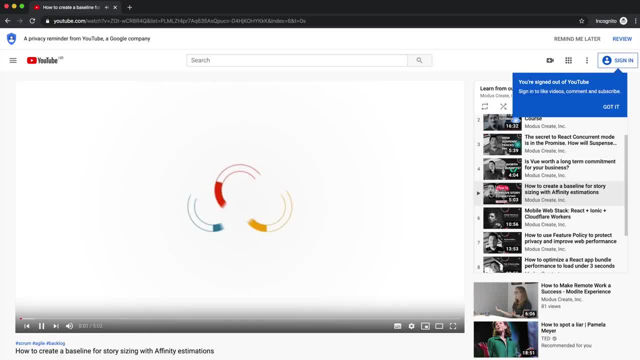 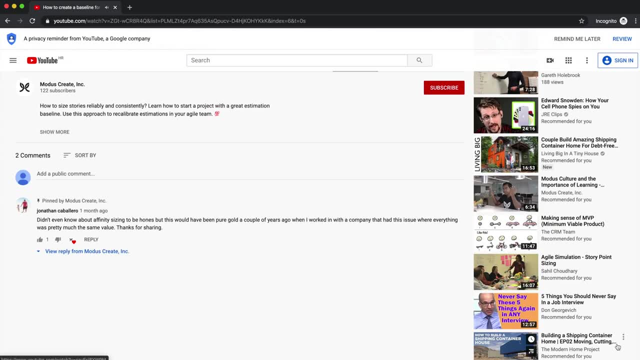 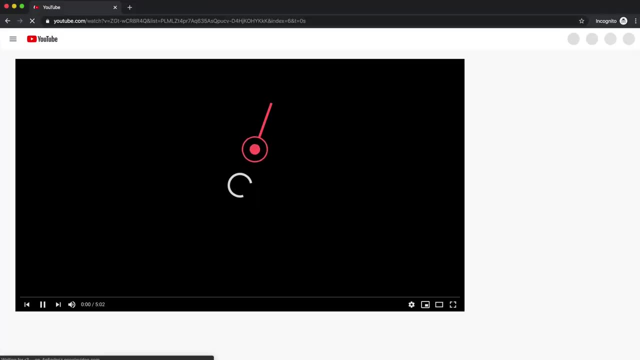 usually start from the top of the page. For example, Amazon and YouTube do a great job at loading comments when a user scrolls down a little bit. Now I don't need to load comments unless I actually scroll down. I want to focus the downloading of my resources to the hero or to the video or whatever. 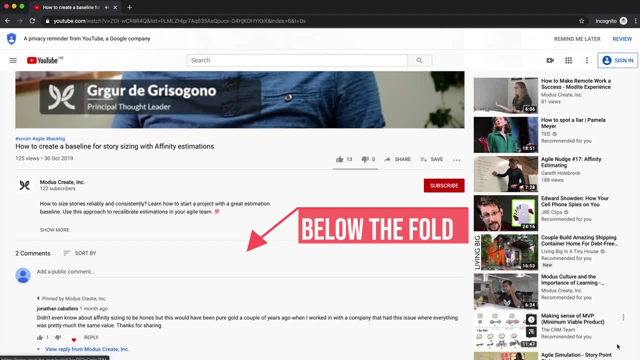 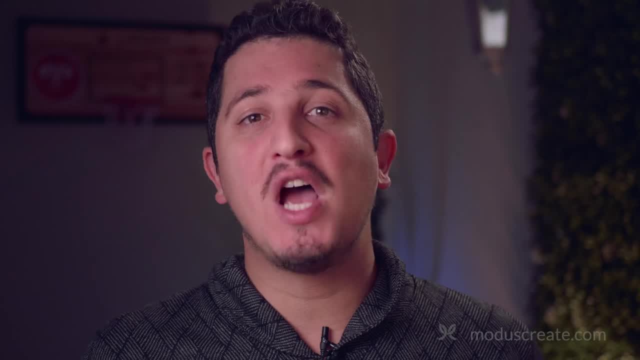 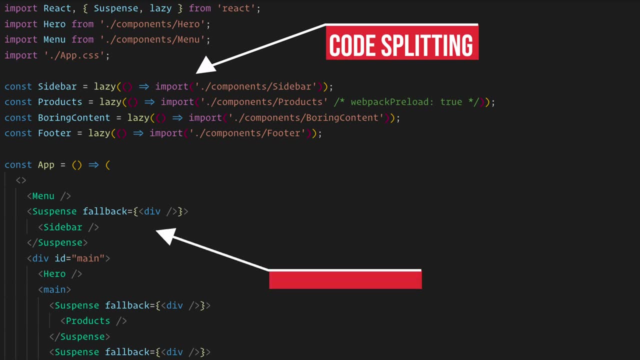 the content is above-the-fold Now. did you know that you can do that with JavaScript as well? You can prioritize downloading of JavaScript resources in your application. With optimal usage of code splitting and lazy loading, you can download just the JavaScript that your users need to see. 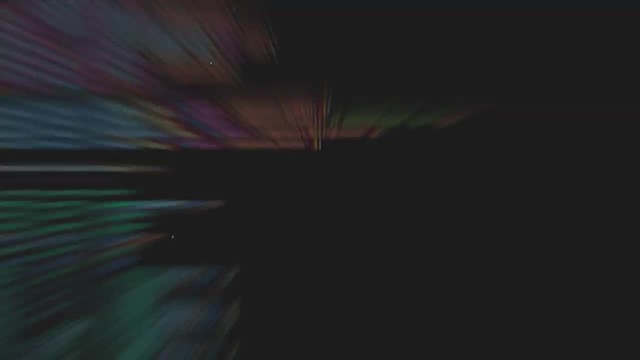 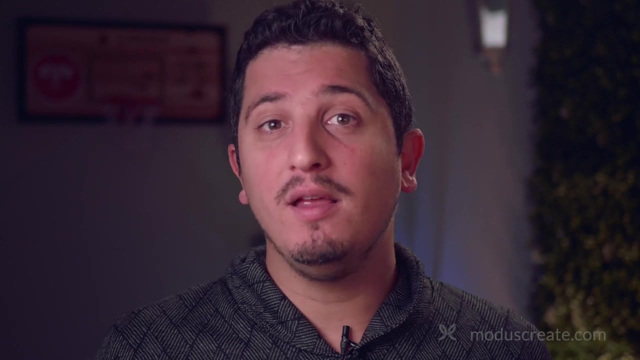 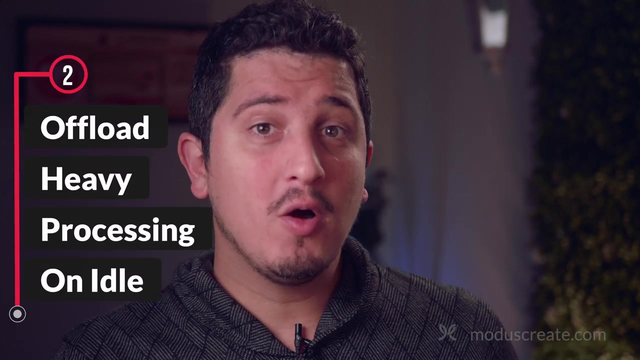 If you want to learn more about how to do that with React, make sure you see my video on loading anything under 3 seconds on 3G. And this leads me to the second valuable decision: Offload heavy work when user is idle. 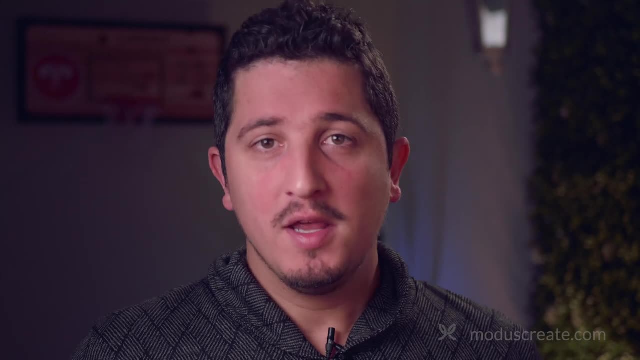 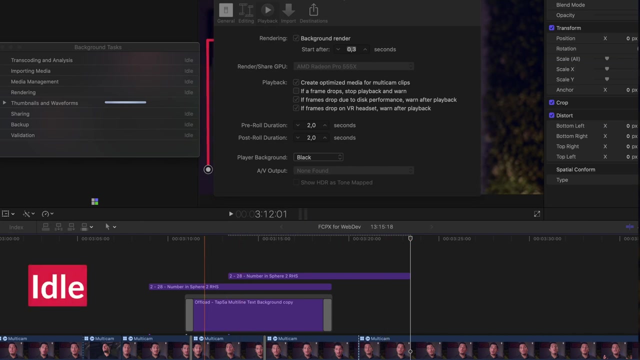 Nothing kills productivity like heavy processing. Final Cut Pro does a great job at that, because it lets me use my timeline and do the work. The background rendering is going to kick in when I'm idle, And when I resume work it's going to pause. This is a phenomenal example how Final Cut 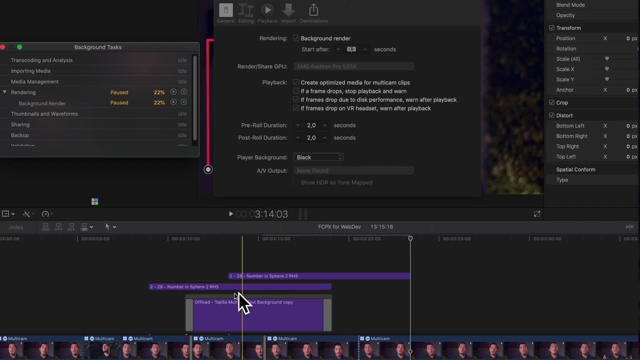 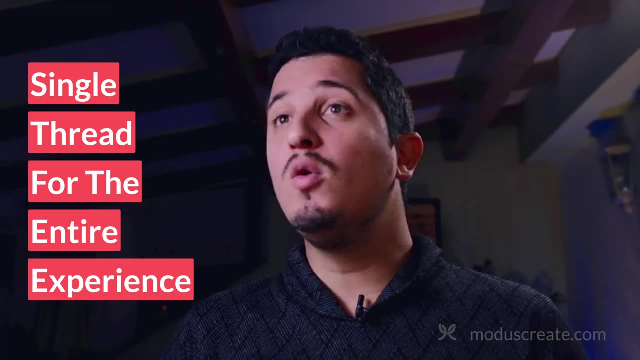 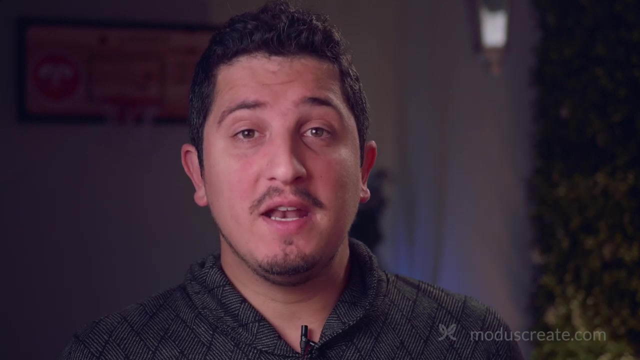 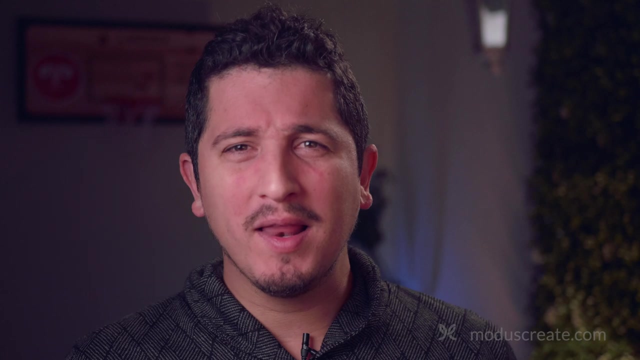 Pro leverages processing when user is idle On the web. this is even more important because we have that single thread that uses the UI, the JavaScript and everything. Interactivity on the web is imperative. Delays in any feedback will make your app look jittery, unresponsive, lagging poor quality. 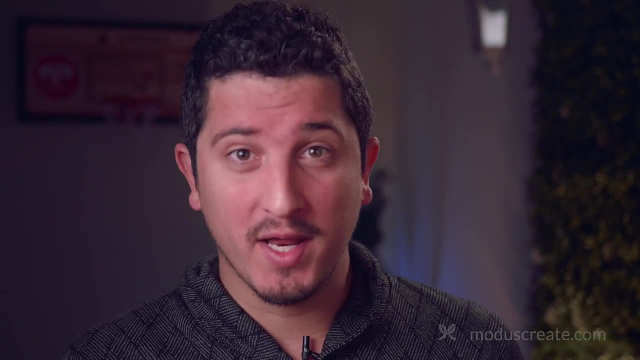 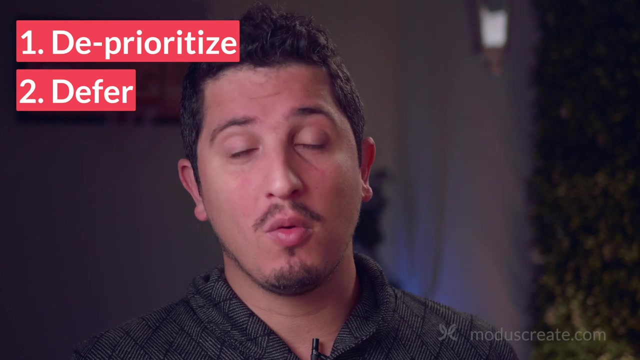 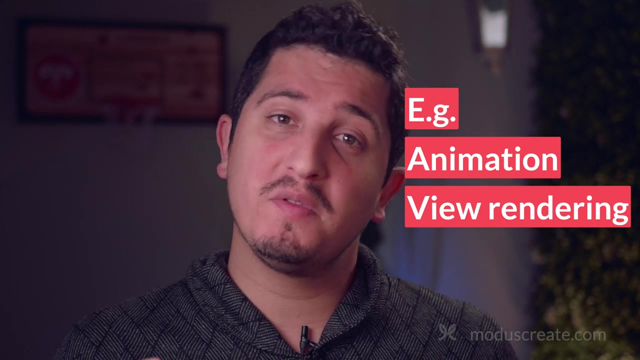 You just don't want that. You don't want it, Your users don't want it. I suggest you pause or defer any activities that are going to use your processor or even the GPU while user needs interaction, And that's things like animation or even view rendering, the parts of the view. that's 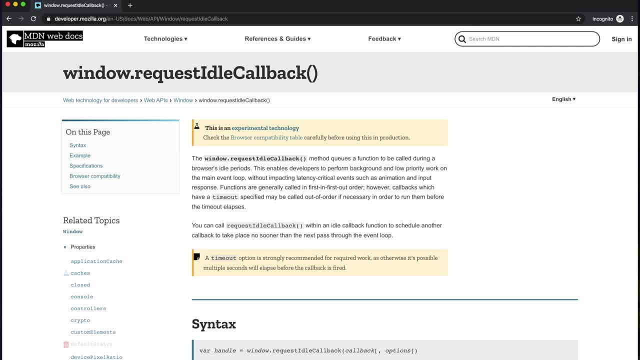 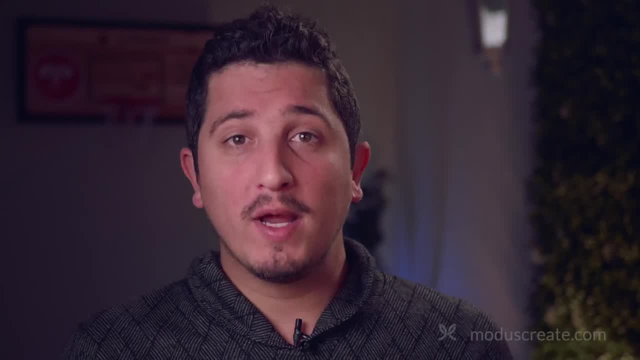 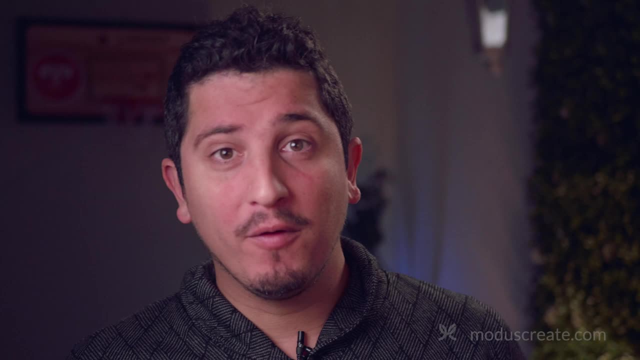 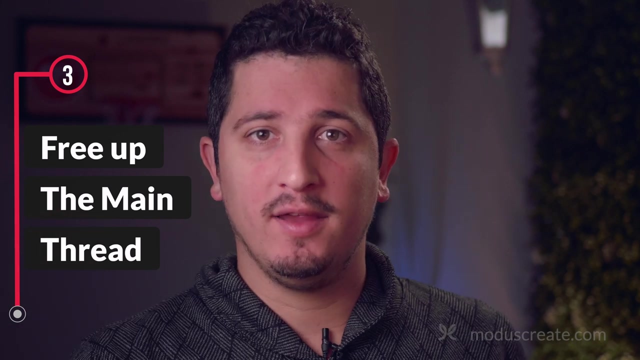 below default. On idle callback, it's a perfect API that you can leverage for this. Doing the work when the user is idle is going to greatly improve the responsiveness of your main thread, But you can also move things out of the thread. This gets us to the point number three. keep the main thread underutilized. 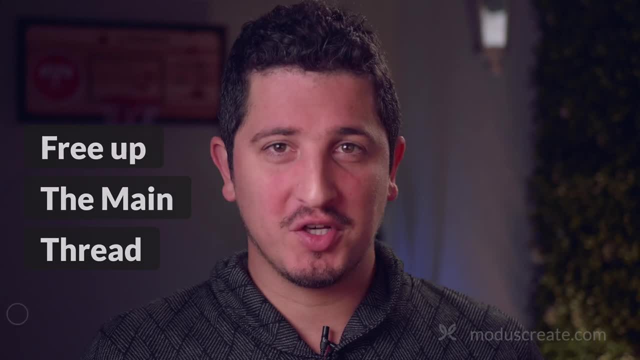 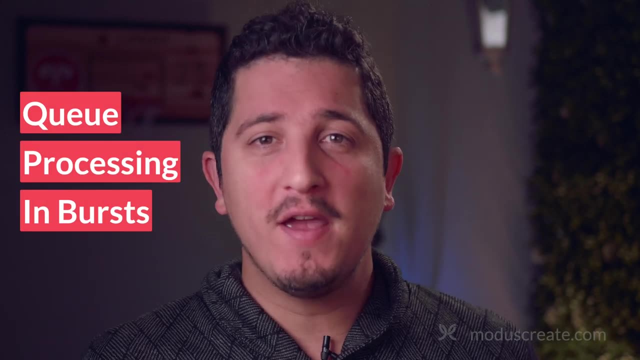 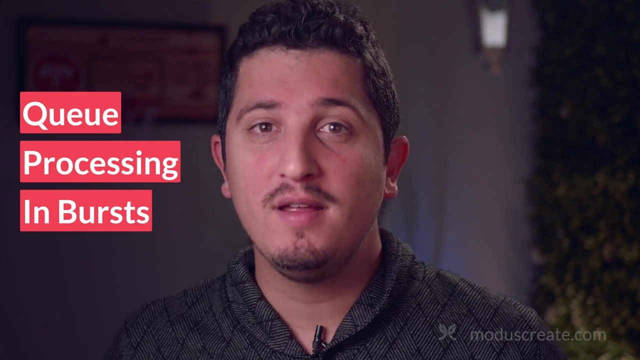 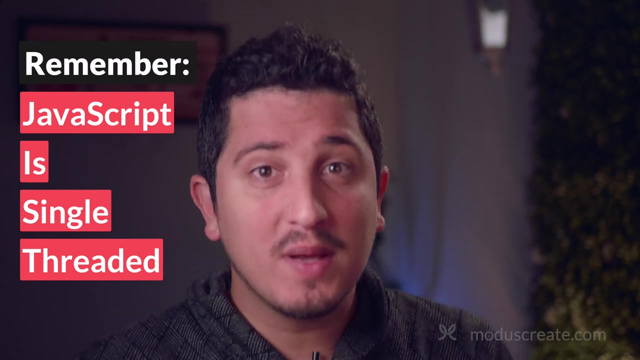 Final Cut Pro prioritizes user interaction. Now, when it needs to do any heavy work, it tries to employ all the possible available processing power. This makes sure that the work that needs to be completed is actually done as soon as possible. Web applications are even more sensitive to processing, especially if they use that single. 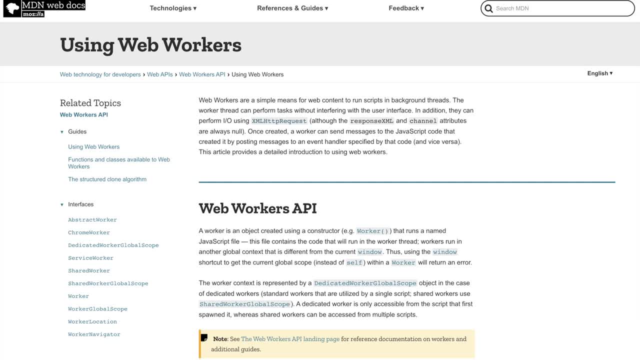 available thread, And that's why we should offload any processing to web workers. This is really an upgrade from moving things around faster and faster. To make it work faster, we're going to need to work on the roadmap. We're going to need to deploy the code in the text editor. It's an excellent way to watch the page. 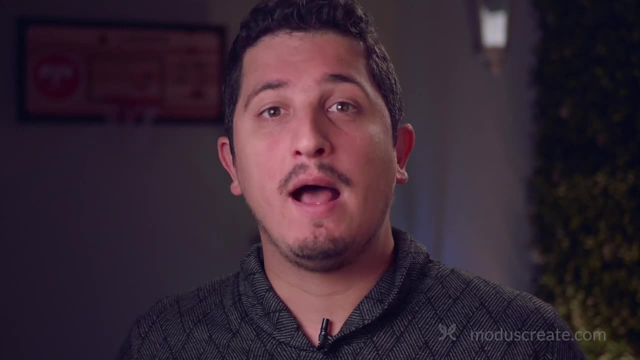 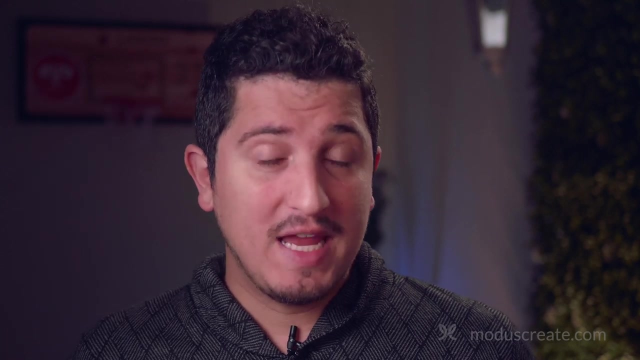 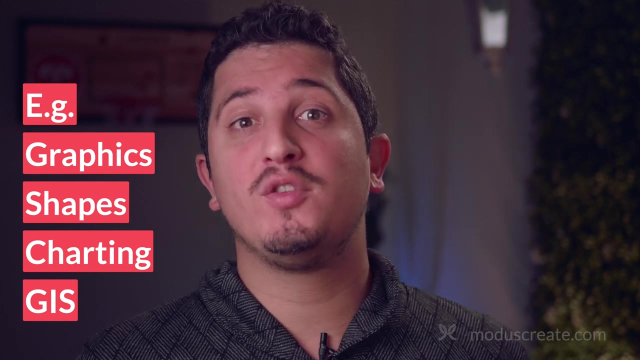 moving things, shifting things to when user is idle. Now you can do things when user is idle and you can offload things in a worker thread. For example, if your application does any graphics rendering, creating shapes or anything advanced with charts and similar libraries, you could use web workers. 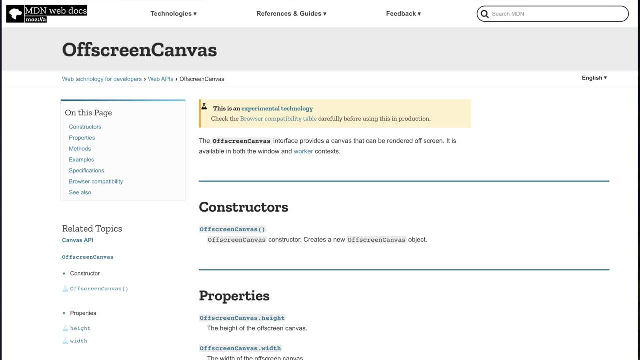 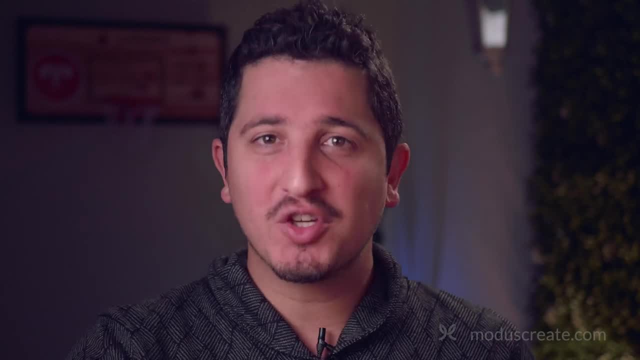 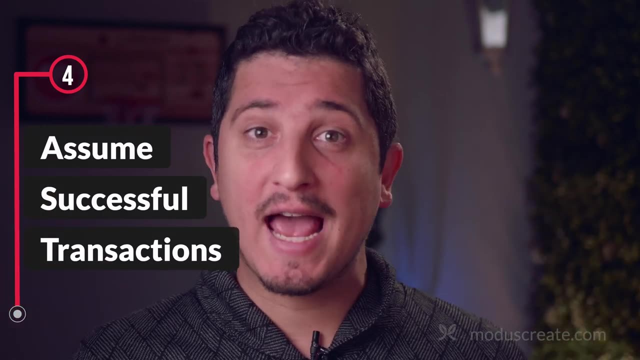 together with off-screen canvas. This will make your application a lot snappier and all the heavy processing will be moved outside the interaction layer with your user. And the final fourth tip is: assume successful transactions, And this is my favorite When I add media to Final Cut Pro. 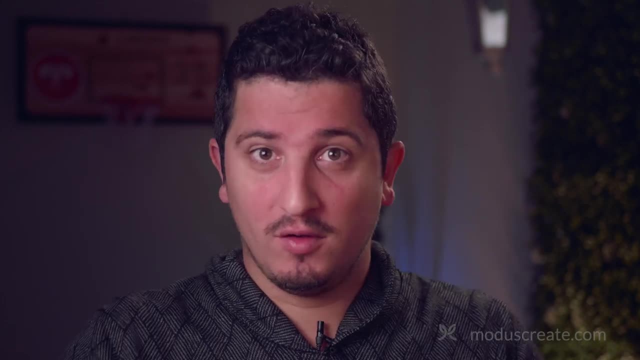 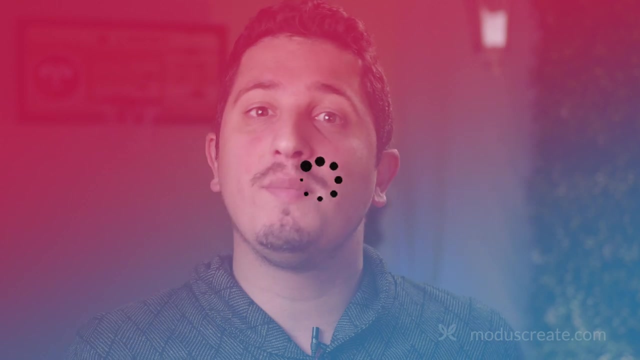 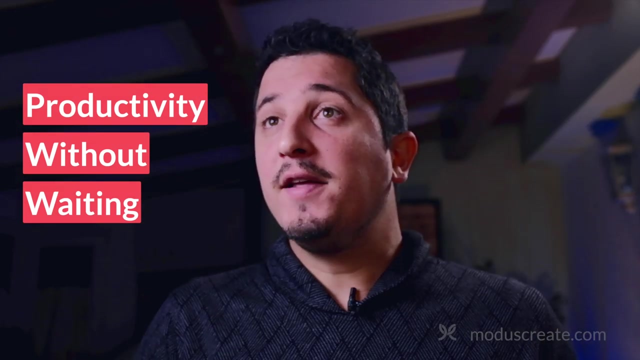 they can usually be many dozens of gigabytes large. but you know what? Final Cut Pro doesn't just show a spinner, doesn't tell me that something is loading, downloading, loading. It lets me use those resources immediately. Final Cut Pro lets me be productive without waiting.